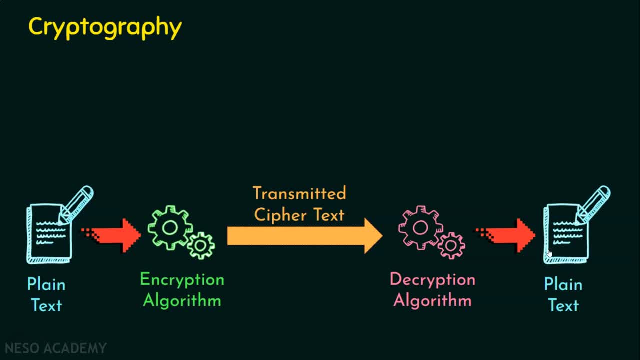 of the decryption algorithm is to convert the ciphertext to its plaintext. Now, in this whole process, if you observe, this encryption algorithm is going to take two important inputs, But here we have seen only one input. What is that? Plain text only. What is the next? 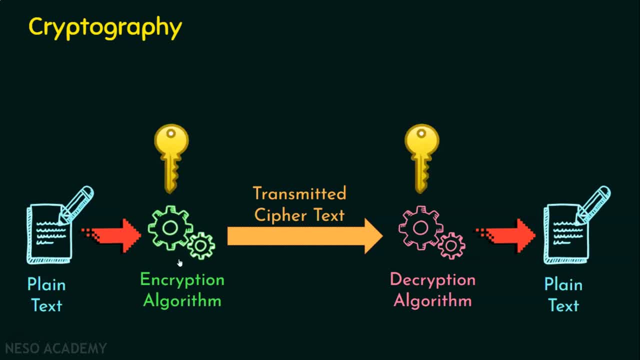 important input. The next important input is the key. So, as mentioned, whether it is an encryption algorithm or a decryption algorithm, it will be taking two things or two input. If it is an encryption algorithm, it is going to take plain text as an input. If it is a 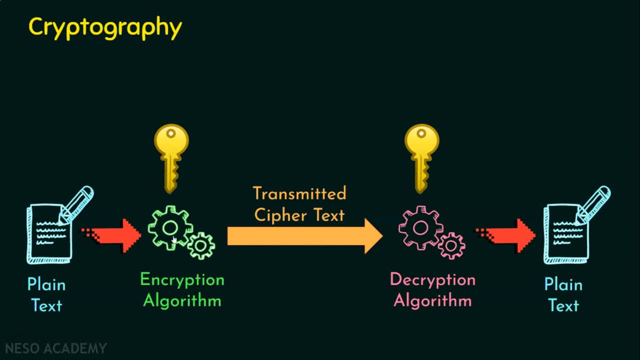 decryption algorithm. it is going to take ciphertext as an input. Now, the second important information that is going to be used by both the encryption and the decryption algorithm is the key. Now, this is the key, which is the most critical information and which should be kept. 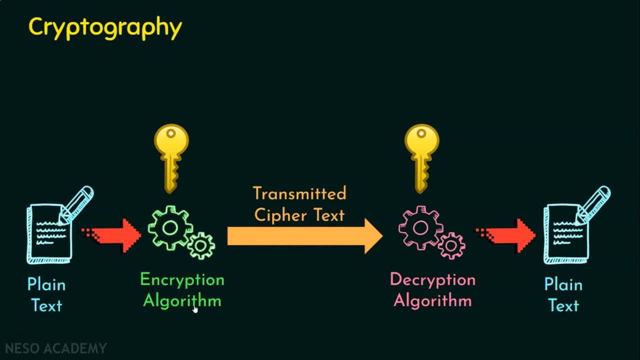 secret. The encryption algorithm will be generally kept public. Public means. even attackers may know what is the encryption algorithm that is used to generate this ciphertext, But the real security should lie in the keys. This key is the most vital and the most critical information that should be. 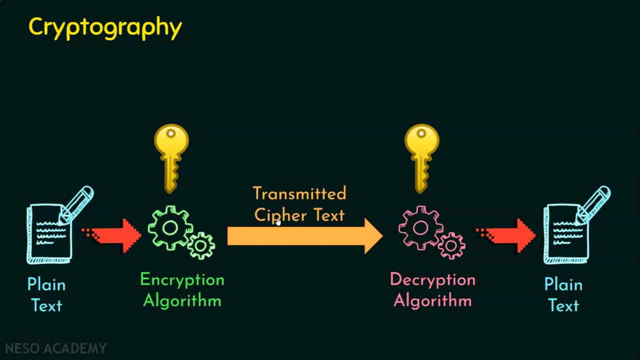 kept more secret than anything else. Suppose if an attacker is able to know what is the plain text equivalent for this ciphertext. this may be a guessing attempt also, But if the attacker knows the key, he can understand all the communication between the sender and the receiver. I hope now you can understand why we need to keep. 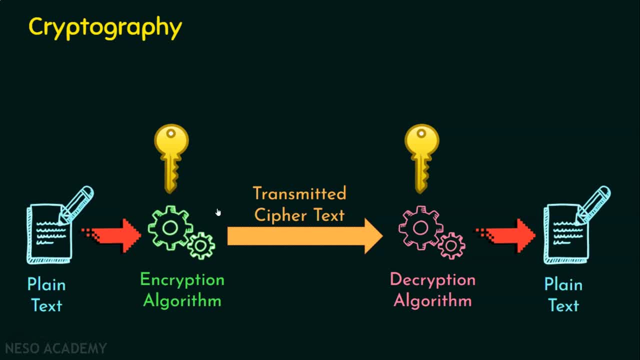 this key more secret and more secured. right From this, we can understand that we are sending or transmitting only ciphertext, not the plain text, because plain text can be viewed by many people on the internet and if it is encrypted or if it is a ciphertext, 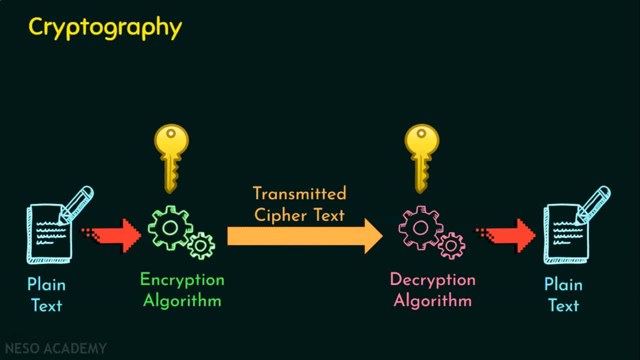 no one can understand or no one can know what the message is, except the sender and the receiver. So we are sure that we are going to send only ciphertext. In order to send the ciphertext, we need to generate the ciphertext, which is done by the encryption algorithm, where this encryption 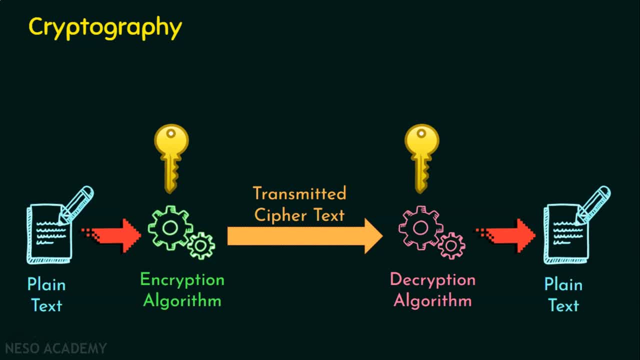 algorithm takes the plain text and the key as an input and produces the ciphertext as an output. Now this ciphertext can be sent on the internet. Even attacker can get a copy of the ciphertext. but we can be very confident that if our encryption algorithm and the keys 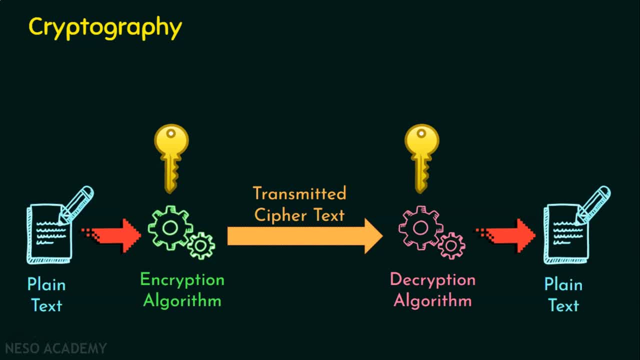 are very powerful. the attacker will not be able to break it because we truly trust the encryption algorithm and the key and receiver. upon the reception of the ciphertext, he can decrypt the ciphertext using the key. Now in the entire process, if the same key is used, if you observe. 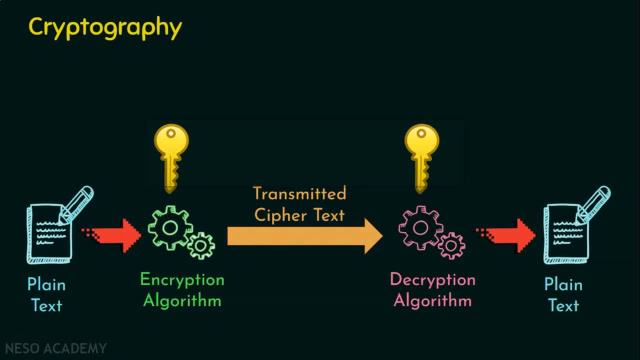 in the scenario I am using the same key for both encryption and decryption. This cipher model- we call it as a symmetric cipher model, because sender and receiver are using the same key and sender and receiver agree upon that they should not reveal the key on any account, So this key should be known. 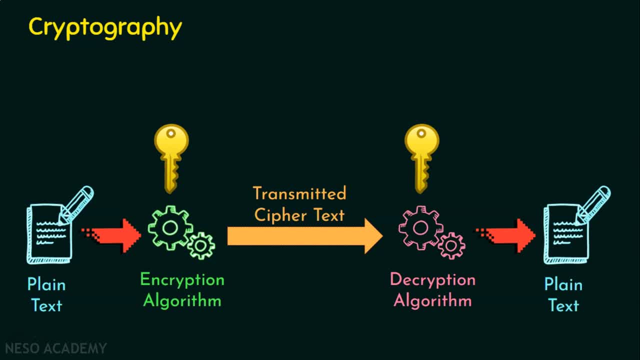 only to two guys: One is the sender and the other one is the receiver. This is exactly the symmetric cipher model is. With this knowledge, let's understand what is cryptography. Cryptography means it is the process of converting the plain text to ciphertext and converting the ciphertext. 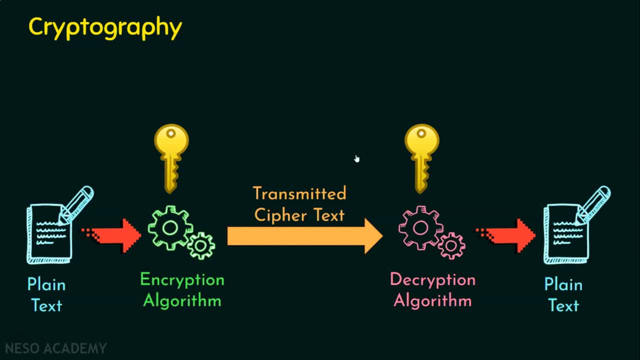 back to its plaintext Now. in this whole process, two important information are involved. One is the algorithms to deal with the encryption algorithm and the other is the encryption algorithm to deal with the encryption algorithm, and the other is the encryption algorithm to deal with the encryption. 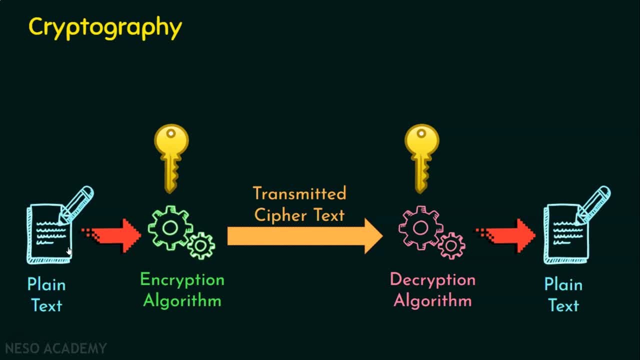 and decryption, and the other one is the key. If sender wants to convert the plaintext to ciphertext, he uses encryption algorithm. If the receiver wants the plaintext back, he uses decryption algorithm. So we will see the definition of cryptography. formally, Cryptography is the art or science. 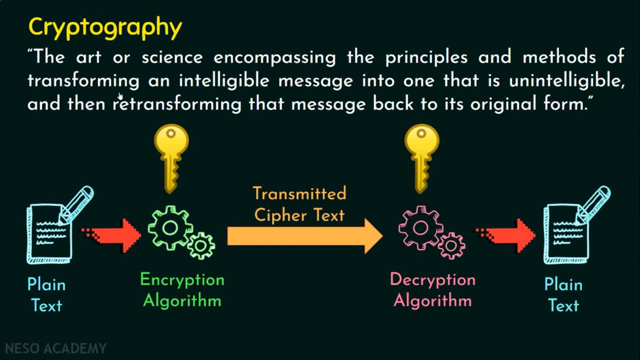 encompassing the principles and methods of transforming an intelligible message into one that is unintelligible. It means cryptography is an art or science that deals with the principles and methods in order to convert the plaintext to ciphertext. Cryptography is the art or science. 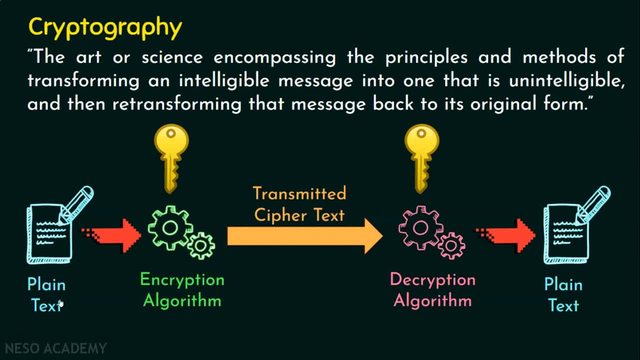 encompassing the principles and methods in order to convert the plaintext to ciphertext. Here, the plaintext is the intelligible message, which can be a readable message. Now we want to convert this plaintext or the intelligible message into an unintelligible one, which is the scrambled text, which is the ciphertext. If someone sees the ciphertext. 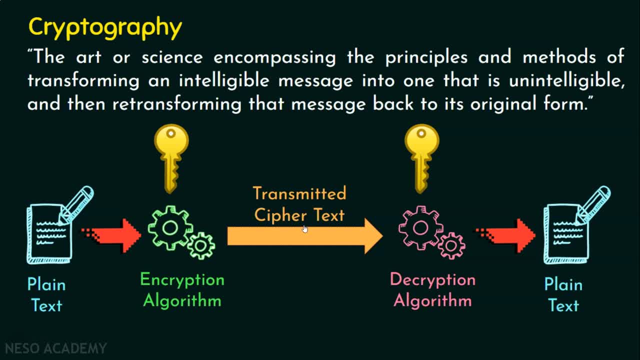 they will not understand what the message is actually because it will be scrambled and it will be unintelligible, So no one can understand what it is. and we will continue dealing with the definition and then re-transforming the message back to its original form When we 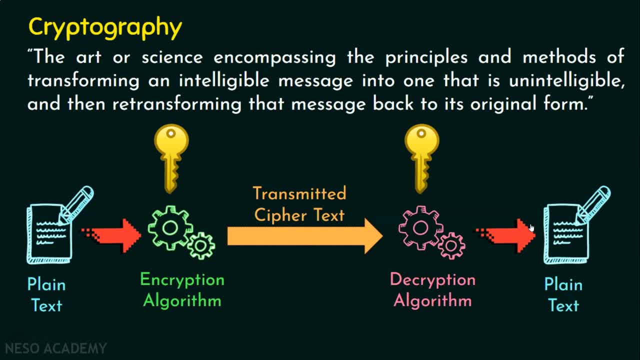 need to re-transform the message back to its original form in the receiver side, because in the receiver side also the receiver will be receiving the ciphertext. only Now the receiver have to give this to the decryption algorithm and this decryption algorithm will be re-transforming. 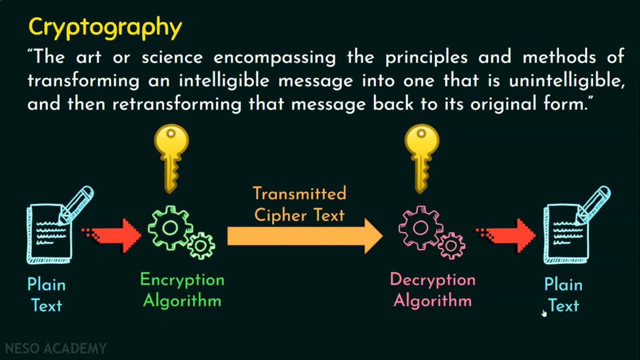 this unintelligible message back to its original form, which is the plaintext form. So this is the definition of cryptography. In the next lecture, we will see about various key terms or key terminologies of cryptography. So we are done with cryptography. Let's now see the two types of 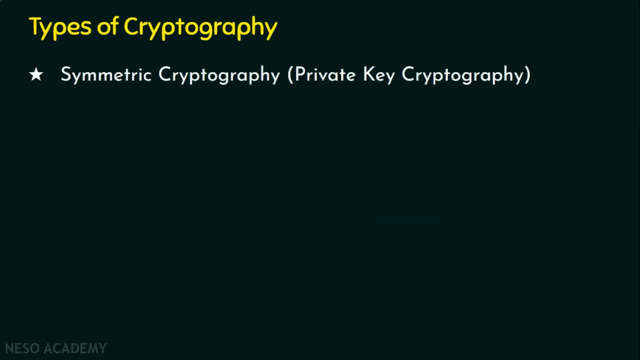 cryptography. Basically, there are two types of cryptography. Number one, the symmetric cryptography, which is also called as private key cryptography, and the next one is asymmetric cryptography, which is also called as public key cryptography. Let's see what is symmetric cryptography and what is. 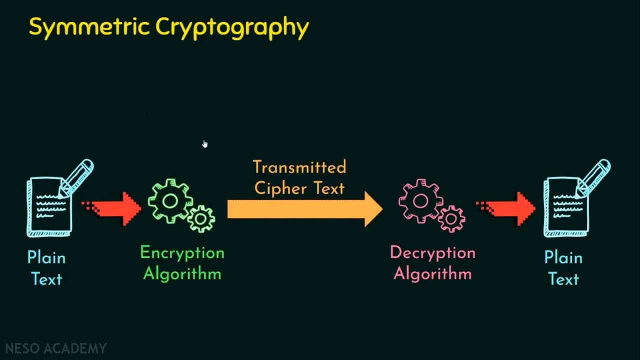 asymmetric cryptography. This is actually the cryptographic technique. is Then, what is symmetric cryptography? In symmetric cryptography, can you see here? the encryption algorithm is using a key, and the same key is also used by the decryption algorithm. So this is the cryptography. 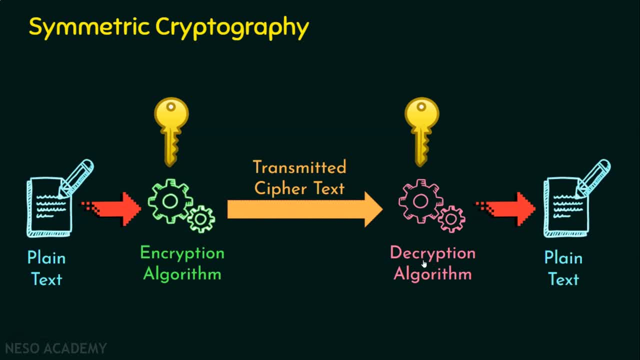 which is used by the decryption algorithm. So if encryption algorithm and decryption algorithm are going to use the same key, then it is symmetric cryptography. Can you see? Same key is used for both encryption and decryption algorithms. In other words, if sender uses a key for encryption. 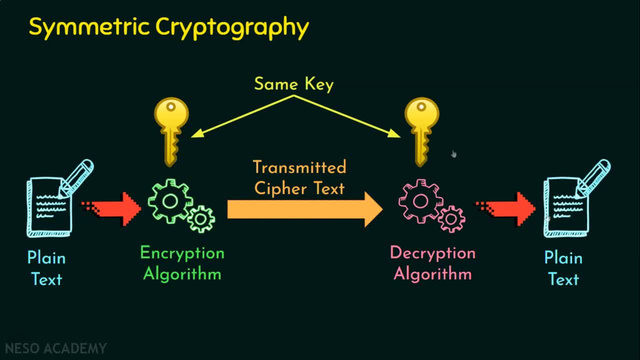 and if the same key is used for decrypting the message by the receiver, then it is symmetric cryptography, which is also called as private key cryptography, because both sender and receiver will be sharing this key and no one else should know about this key except the sender and the 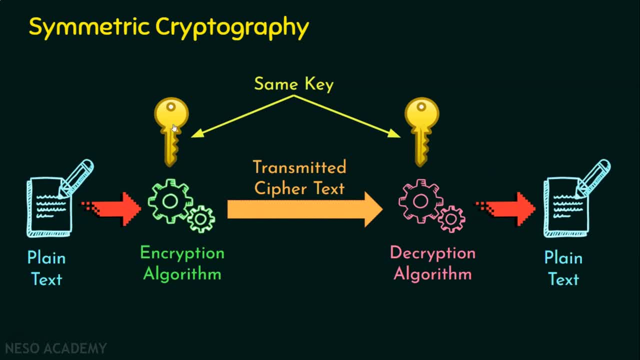 receiver. No one should know the key. Only then it will be secure. So this is actually symmetric cryptography. I will give you a simple example. Say if the key is 100. If sender is using this key 100 for encrypting and if the receiver is also using the same key- 100- for decrypting, then it is. 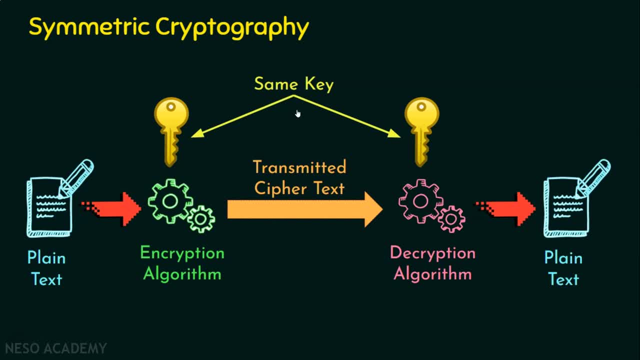 called as symmetric cryptography. Actually, 100 is a very small value which can be easily broken. Actually, cryptographic algorithm uses a bigger number which will not be even readable by humans. The numbers only will be powerful on the internet, and it will be powerful and it will be protecting. 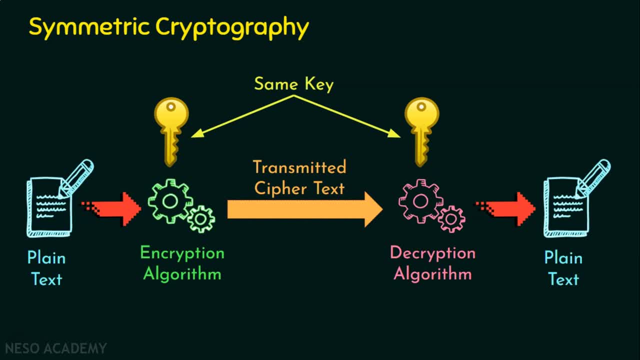 against attacks, because our intention is: attacker should not break the key. Since the key is kept private between the sender and the receiver, this symmetric cryptography is also called as private key cryptography. We are done with symmetric cryptography, Let's now move on to asymmetric. 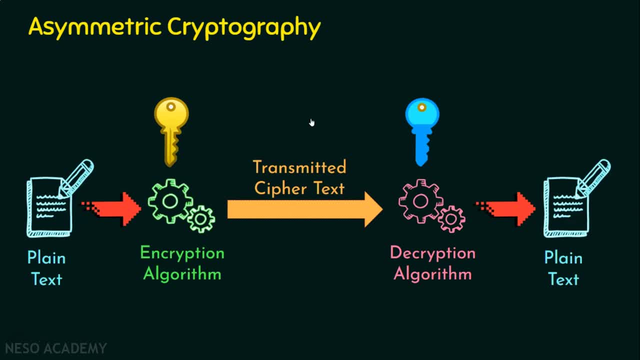 cryptography. Can you see here? Is there any difference when compared to symmetric cryptography? Yes, Can you see here? This is a different key, where this is the key which is used for encryption algorithm and this is a different key which is used for decryption algorithm. 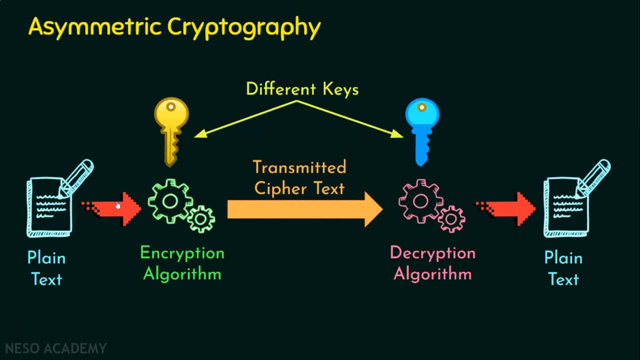 So asymmetric cryptography means if sender uses a different key for encryption and receiver uses a different key for decryption, then it is asymmetric cryptography. Now you may be asking me a question: Is that practically possible? For example, if sender is using 100 as the key? 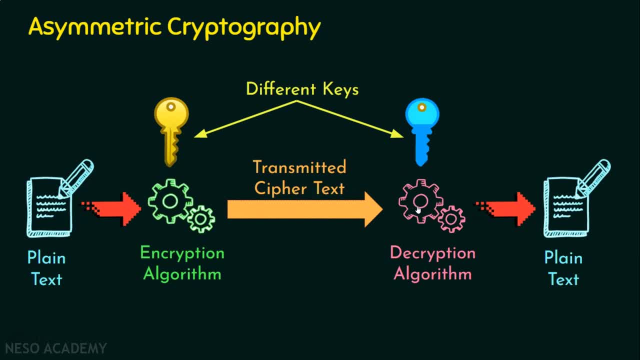 to encrypt the ciphertext and if receiver uses 500 as the key to decrypt the message? is that possible, Because encryption is done with 100 and decryption to be done with 500.. That can be possible if the underlying mathematical concepts are satisfied. Please make. 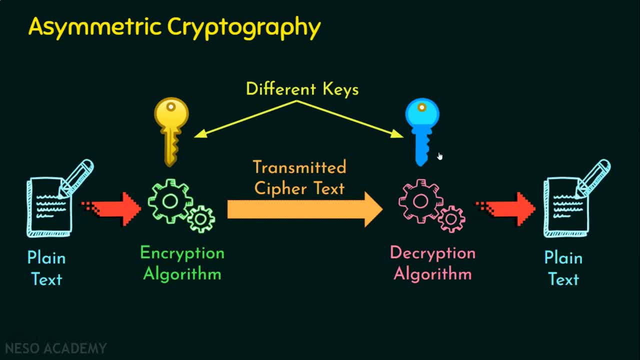 a note of this: Cryptography deals with a lot of mathematical terminologies. The underlying mathematics is more important, So these keys are generated by the mathematical algorithms in order to deal with the cryptographic techniques. You will understand this when we see some examples. 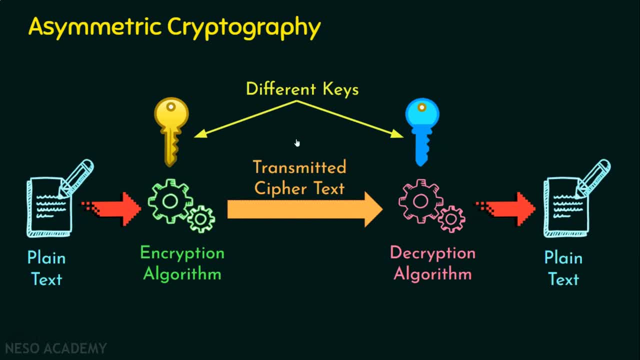 and live demos For time being. just understand: if sender and receiver or if encryption algorithm and decryption algorithm are using asymmetric cryptography, And that's basically the same, the same key, it is symmetric cryptography. If encryption algorithm and decryption algorithm, or if the sender and receiver uses different keys, then it is asymmetric cryptography, Since we have 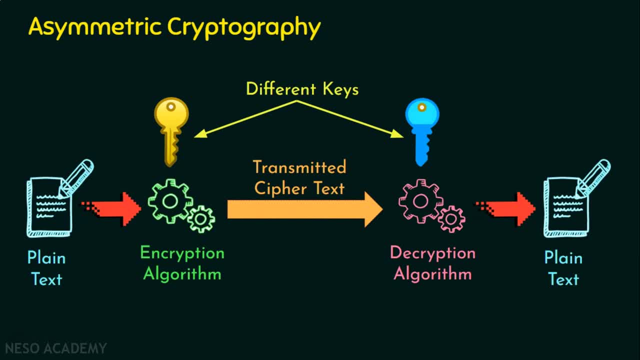 two different keys here. one key is named as a public key and the other key is named as a private key. So here I didn't mention which key is a public key and which key is a private key. Anyway, we will be understanding this in the upcoming lecture. what is a public key and what is a 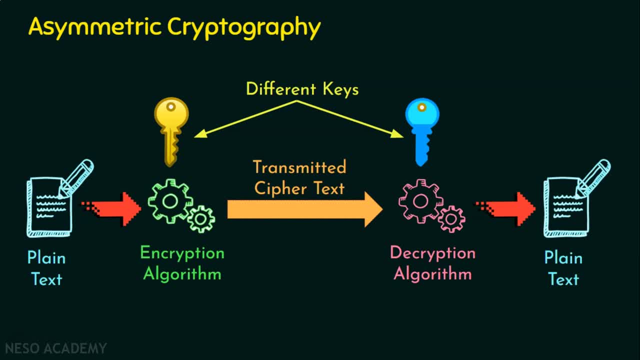 private key. For time being, just understand two different keys are used. One is a public key and the other one is a private key. When we have public key and private key, then this asymmetric cryptography is called as a public key cryptography. When both the keys are private, then it is a 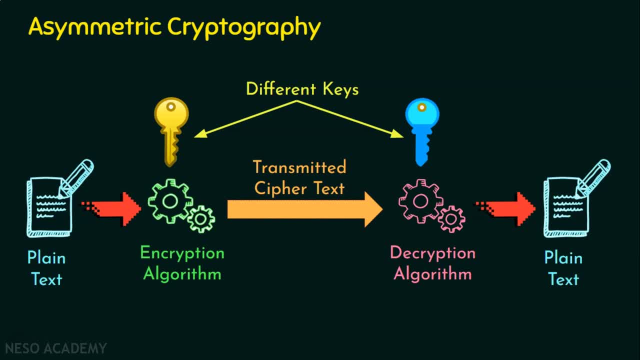 private key cryptography or symmetric cryptography. We are done with symmetric and asymmetric cryptography. Let's now see about this encryption schemes. Generally, this encryption schemes are very important and this decryption schemes are the reverse of the encryption schemes. Let's talk about the encryption schemes now, because in order to generate the ciphertext, we need to 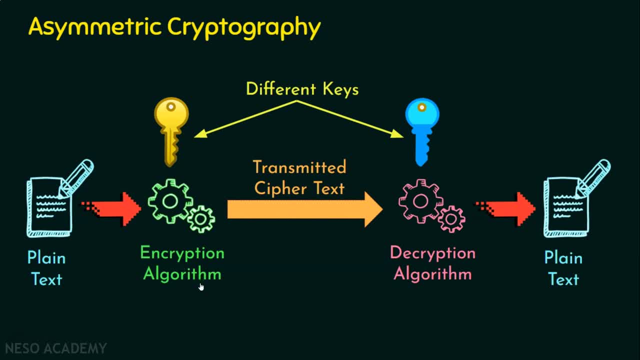 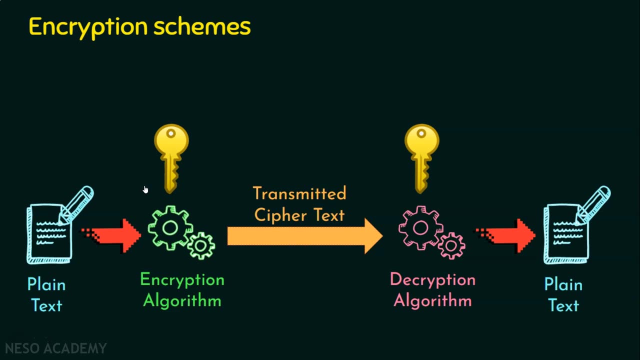 need encryption algorithms or encryption schemes, and we are going to see about two important properties any encryption algorithm or encryption schemes should possess. Let's see that now. Let's take this example. Don't worry whether it is a symmetric encryption scheme or asymmetric encryption scheme. Just imagine it is an encryption scheme. Now what are the two qualities? this? 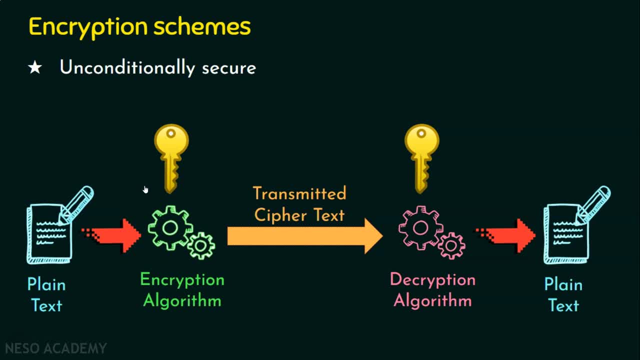 encryption scheme should have: Number one: it should be unconditionally secure, and number two: it should be computationally secure. Let's focus on unconditionally secure. Now, when you will call this encryption scheme or encryption algorithm is unconditionally secure? I will give the answer now. An encryption scheme is said to be unconditionally secure if the ciphertext 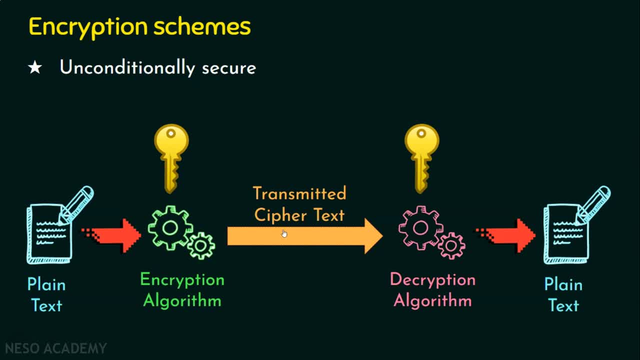 that is generated by this encryption algorithm or encryption scheme does not contain enough information to determine uniquely the corresponding plaintext, no matter how much ciphertext is available. For example, if there is an intruder here or an attacker here, he gets the ciphertext If the attacker is. 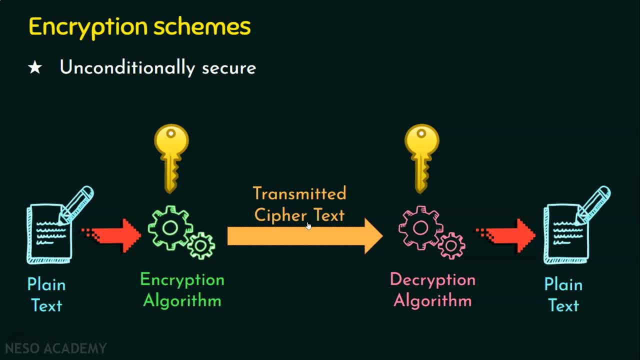 able to guess what is the plaintext equivalent to the ciphertext based on the quantity of the ciphertext that he has. If the attacker is able to guess what is the plaintext equivalent to this ciphertext that he has received, then it means the encryption algorithm is not unconditionally secure. When you 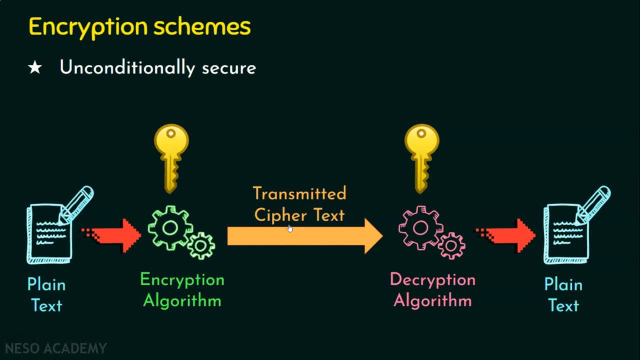 will say it is unconditionally secure. if an attacker receives the ciphertext- and he has received a lot of ciphertext and still he is not able to determine what is the equivalent plaintext, then we will call this encryption scheme as unconditionally secure. So the attacker has received a lot of ciphertext, but still he is not able to determine what is the. 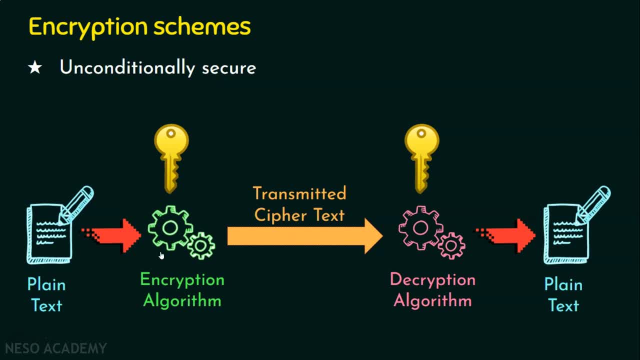 equivalent plaintext. This ciphertext is generated actually by this encryption scheme or algorithm only, and that's why we are referring it as unconditionally secure. We are done with unconditionally secure encryption schemes. Let's now see the second one, which is the computationally secure encryption scheme. When we will call this encryption algorithm or 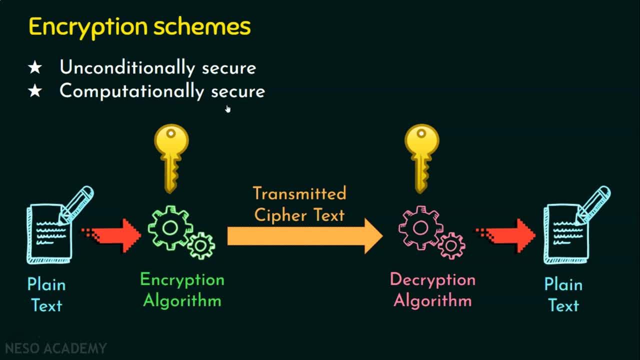 encryption scheme as computationally secure It is, depending on two factors. Let's assume the attacker is receiving the ciphertext and if the attacker is investing a lot of time in breaking the ciphertext. and the attacker is investing a lot of efforts to break the ciphertext but still he is not successful.